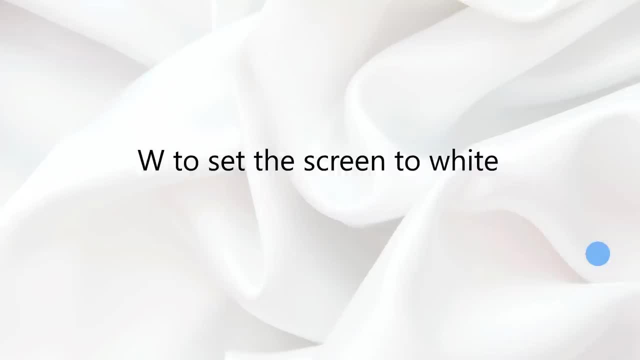 5 or the function 5 key to jump into presentation mode. and that's going to bring us to our very first shortcut key that you could use while presenting in PowerPoint. You could press the W key on your keyboard and that will shift the slide to white. 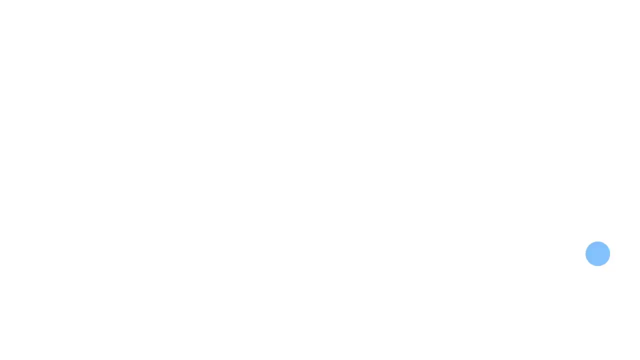 So I'm going to go ahead. let's press W, and here you see it, my slide is white Here I'll press it again and that will bring me back to the slide that I was on. Now, this is very effective if, let's say, you're presenting some content and then you want 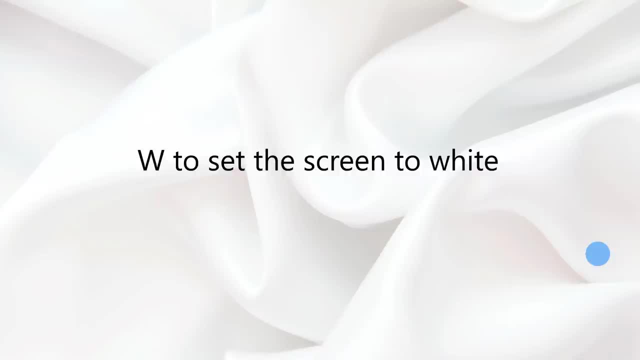 your audience to focus on you instead of the slide. you could shift that focus. Also, a presentation I attended a few years back. the presenter used this very effectively, where she threw up an image of a website design and there had been a change to the website. 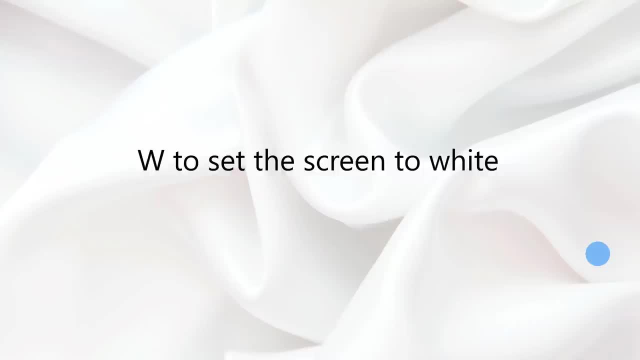 design that we all had previously known. and what she did is she put it up for an instant, she hit the W key to hide it and then we had to guess what had changed with it. So kind of a neat technique that you could use while presenting and, like I said before, 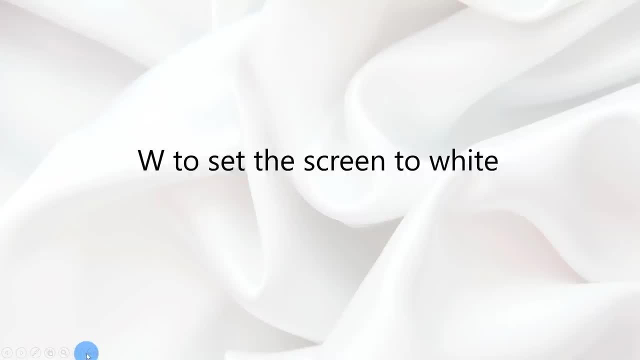 in the intro, One thing you could do. As I move my mouse here, you see all these controls appear at the bottom. If I click on this menu, I could go to screen, and here too I could indicate that I wanted to shift to a white screen. but then again I have to pull up this menu, I have to fumble. 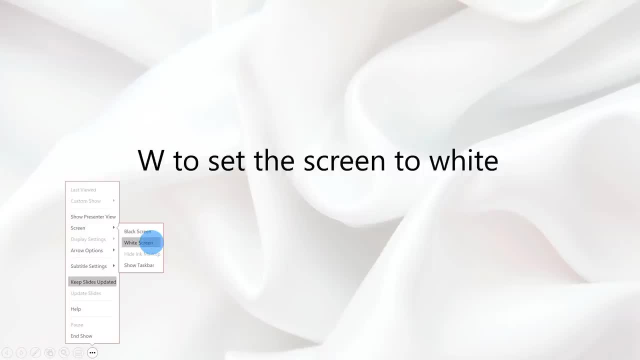 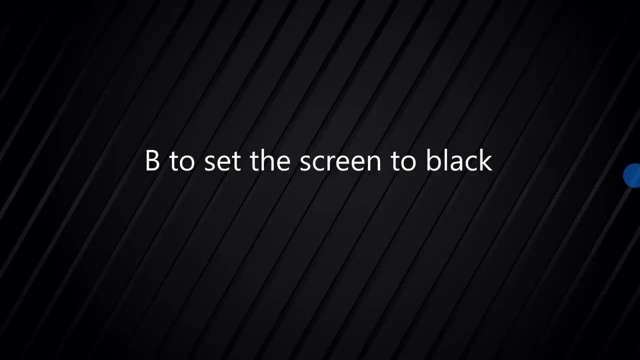 through it. Using shortcut keys is simply much more effective and streamlined, especially when you're presenting in front of an audience. And that brings us to our next one. So not only can you shift the screen to white by pressing W, you could also press B to toggle. 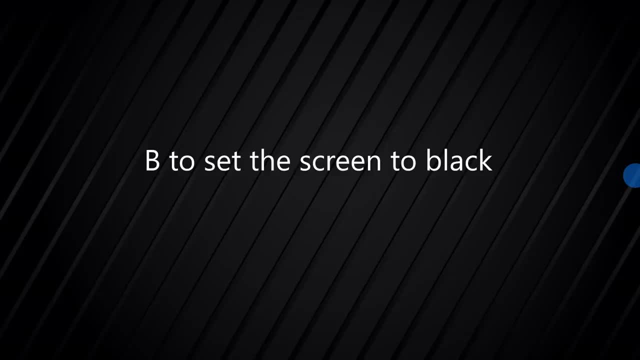 the screen to black, So you effectively turn off the screen. You can also turn off the presentation, and then here I bring it back by pressing B again. So another nice way to have the audience focus on you instead of the content. You could choose whether you want to use W or B, depending on the color that you want. 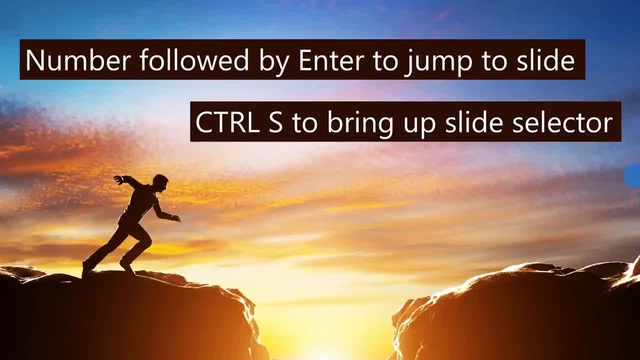 Now, this next one is a fun one. What you could do is oftentimes, when you're presenting, someone might say, oh, could you go back to this slide or could you go back to that slide? An easy way to jump around your slide deck is you simply press the number of the slide. 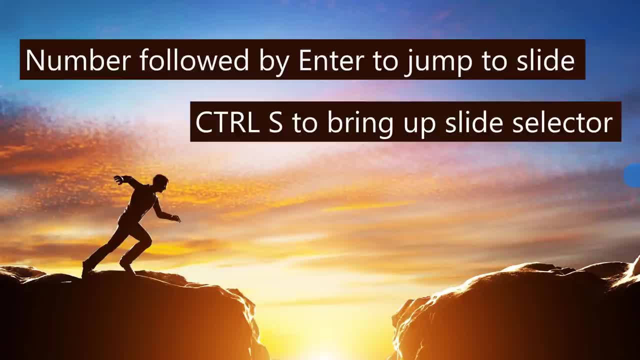 followed by the enter key. So if I want to go back to my first slide, which was about turning the screen to white, I press 1 and then enter, go to my second slide, 2 and enter and back to the third. 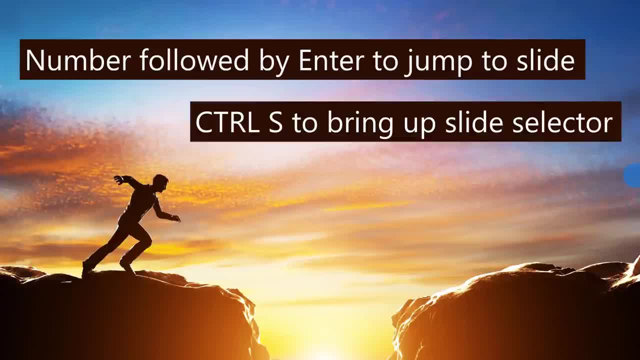 slide 3 and enter. Another way I could also jump around in my slides. if maybe I don't remember the particular number, I could press control S and that brings up all my slides. especially if I title my slides something more descriptive than slide 1, I could very easily find the slide and 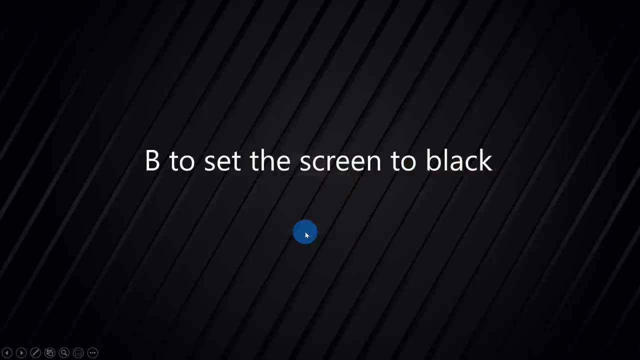 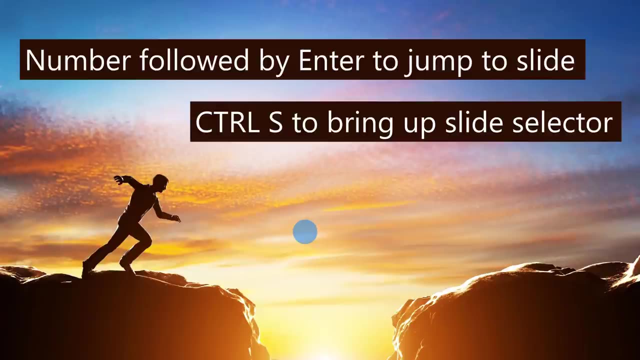 let's say I want to go back to 2, click on go to and then I'll jump back to that slide. So the slide selector is also a very nice way to navigate throughout my presentation without having to click through all of the slides. 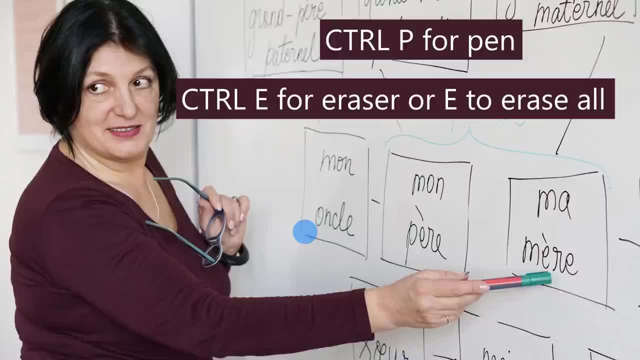 Now the next one. this is a fun one to be able to mark up your slides. So let's say that here's a teacher and she's teaching French uncle, father and mother. Let's say, I want to annotate this slide. 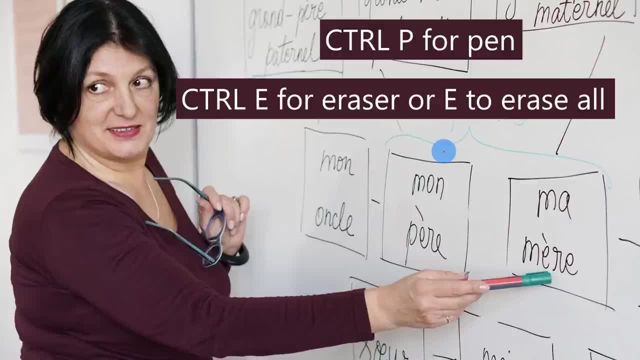 I press control P. The reason we're pressing P is because P stands for pen, and then I can annotate the slides. So maybe I say: okay, class, make sure you pay attention to this, And you want to have the mob, because that's my, and so, whatever your talk, track is along. 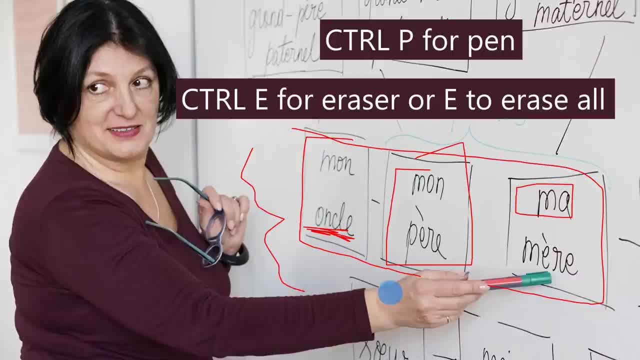 with your slide, you could insert that on, And so here I'm adding a whole bunch of markup, And if you press control E- E for eraser, that'll bring up the eraser tool, and then I could delete parts of my markup. 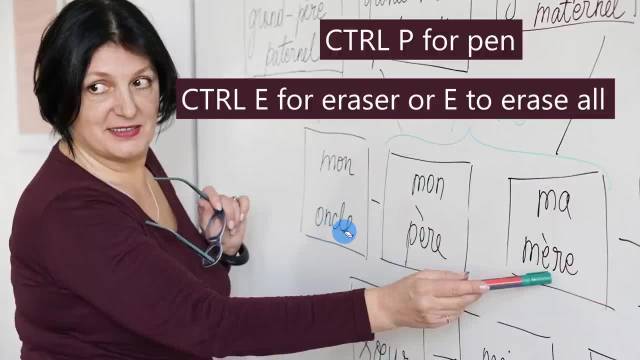 But let's say I really just want to delete everything or erase everything. I could press E and that'll get rid of all of my markup on the slide. Now you see, I currently have the eraser. If I want to get rid of the eraser, I simply press control E again. 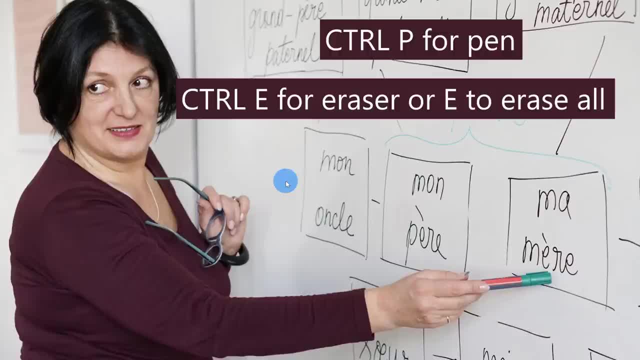 And that'll send me back to my arrow. Similarly, if I'm on control P and I no longer want to annotate, I simply press control P again and then it returns back to the mouse. So quick way to annotate your slides. some other controls that you could also use to: 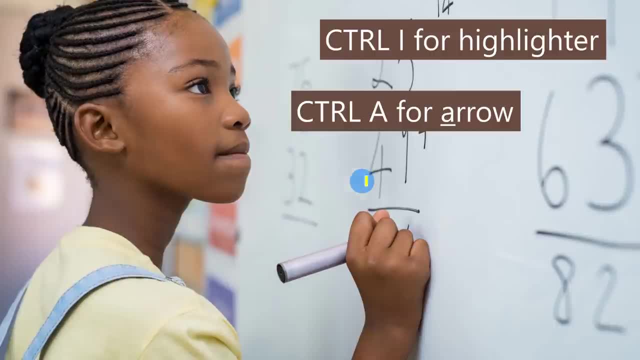 annotate your slide. You could press control I and what that'll do is that brings up the highlighter. So let's say this: uh, this lady here is writing on the whiteboard and maybe I want to highlight the 82 and say: Hey, class, pay attention to this area down here. 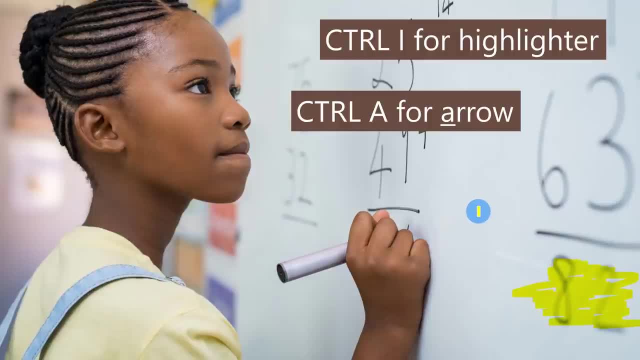 I could highlight it and if I want to bring my arrow key back once again, I could press control I again, and that will toggle off the highlighter and control a if I want to bring my arrow back or control a. and there it is Now the reason that I goes with highlighter. 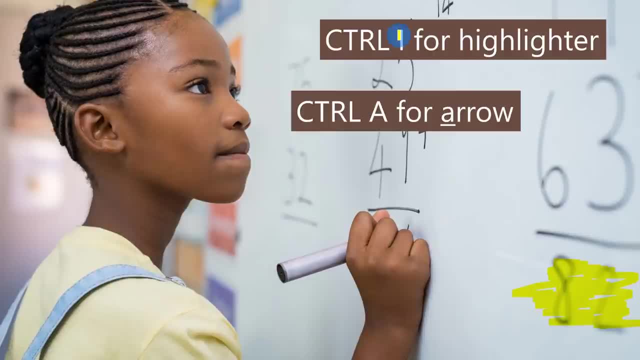 So if I bring it up, you'll notice that the highlighter is a straight line. It looks similar to an eye. So that's an easy way to remember that I goes along with highlighter because it looks like the highlighting tool. So I'm going to go ahead. 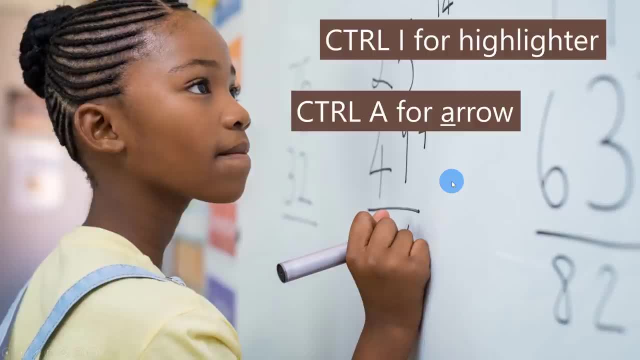 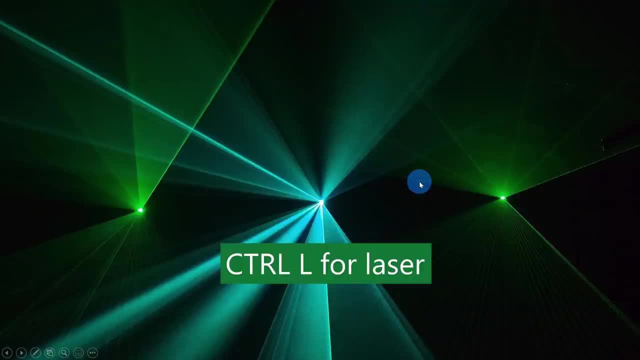 Let's bring the mouse back, and here too, I could even use E to erase everything, or I could press control E to bring up my eraser tool on the next one. One thing that people frequently like doing in a presentation is: you want to point out? 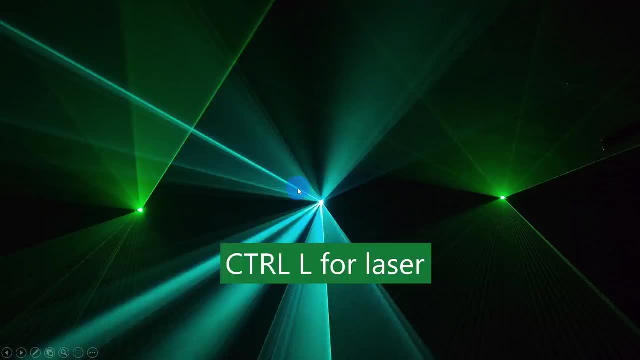 different areas of your slide, or you want people to focus on certain areas and you could use the laser pointer. control L brings up the laser pointer and so here I have a red laser pointer and I could say: Hey, using my laser pointer, and look at this laser look. 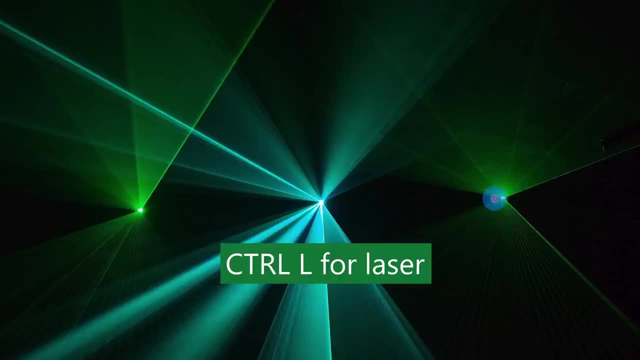 at this laser: It's a blue laser. And then look at this: This is a green laser. This is a green laser. So I could use a laser to call out a laser. kind of reminds me of inception. I have this blue halo around. 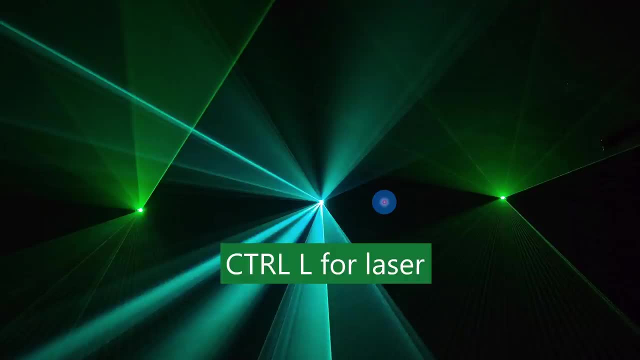 This is a cursor highlighter- highlighter that I'm using. that's unassociated with the PowerPoint, but just to help you know where I'm pointing. and then here too, if I want to get rid of the laser, I press control L. that'll return me to the mouse. 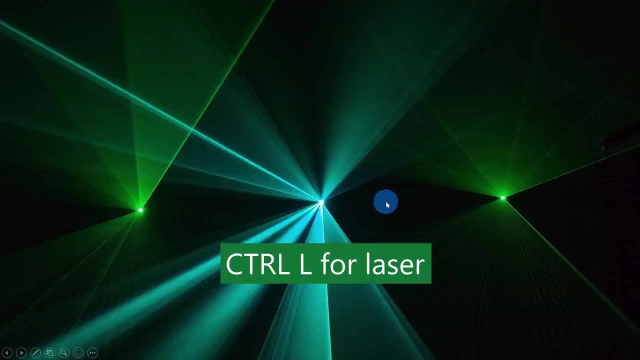 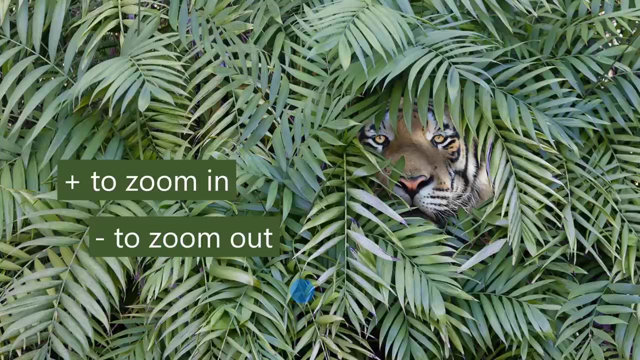 If I click control L again, I could also press control a to bring my arrow key back. So another shortcut key that I can use now. one of my favorites is: let's say, you're showing a slide here and can everyone find the tiger in this photo? 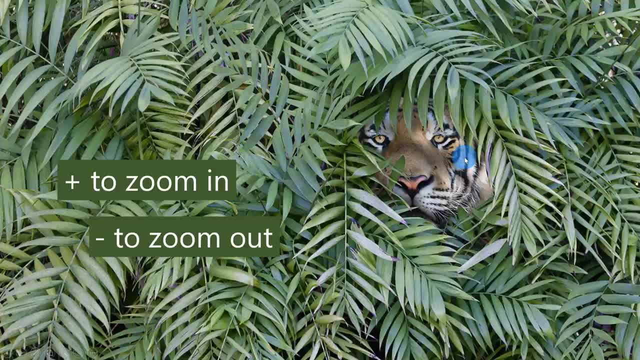 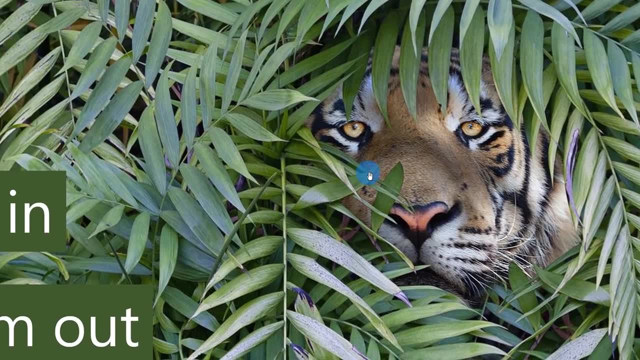 If not, maybe I could zoom in and that might help. All I have to do is press the plus key on my keyboard and that will zoom me in, and then I could use my mouse to pull around the zoomed image or to pan around the image. 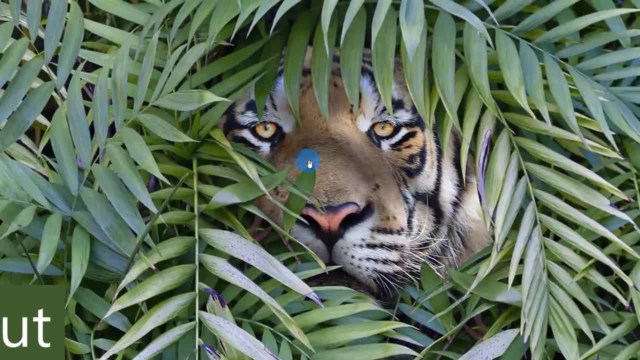 So here I am. that's as far as I can zoom in, and hopefully all of you can see the tiger now. If you, if you still can't see the tiger, I don't know what to say. I won't be able to help you. but that's as close as I can get. 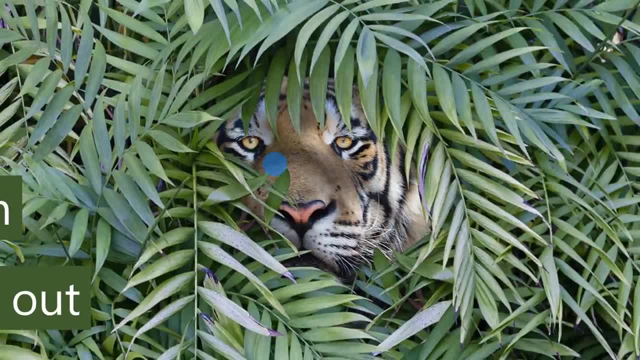 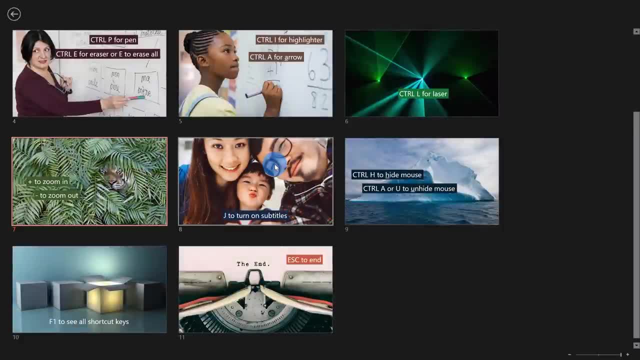 Now let's say you're all zoomed in. Yeah, You can pull back out. you could press the minus key to zoom back out, and here I'm zoomed back to the original state. If I keep zooming out, though, I could continue zooming out, and if I zoom out, all the way. 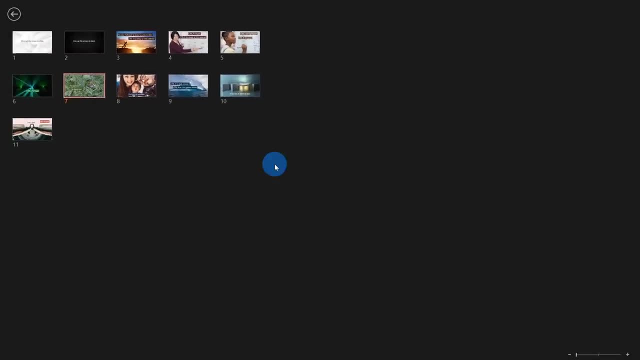 this will bring me out to the slide sorter and I can even zoom out even more to make my slide sorter smaller and smaller, and that's as far out as I can zoom. And once again I can zoom back in, or here I could click on the slide I want to go to. 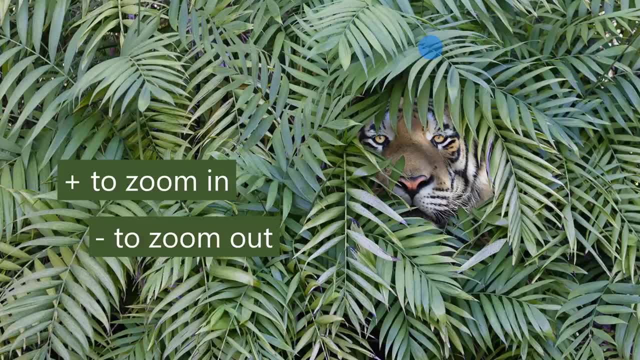 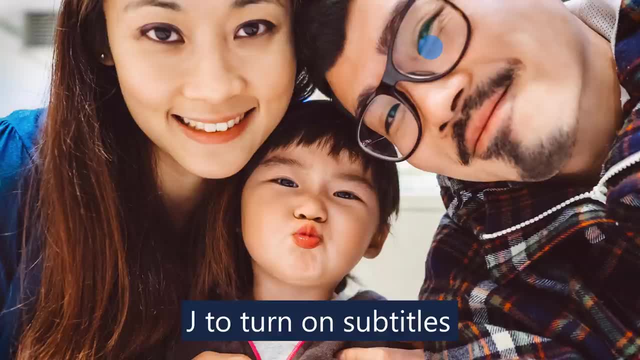 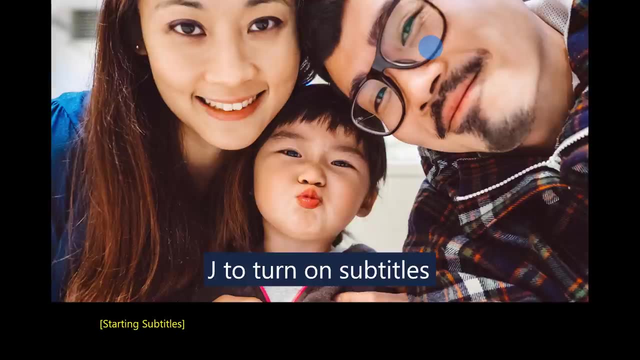 So this is another way to quickly navigate to slides in your presentation, So I'm going to jump back into this slide. Another nice one that's new in PowerPoint is the ability to show subtitles as you're presenting and to turn on subtitles. What you do is you press J, So I'm going to hit the J key and you see down below it says: 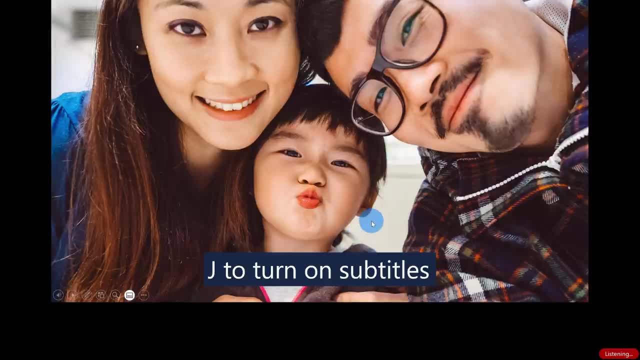 starting subtitles. If I continue speaking, you will see my text appear on the screen. Let's see how good of a job it does at transcribing what I'm saying. All right, Wow, That actually did a pretty good job at transcribing. 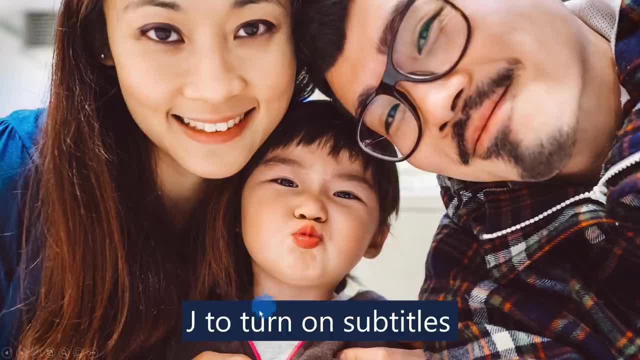 Let's see. Okay, I'm not transcribing my text, But just hit the J key to turn on subtitles and you could press J again to turn off subtitles. And in the settings, before you turn on your presentation, you have the ability to select. 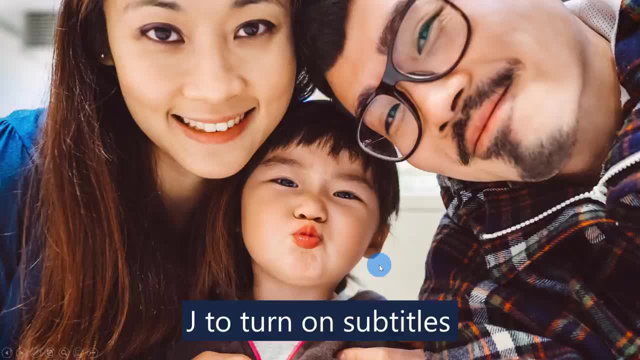 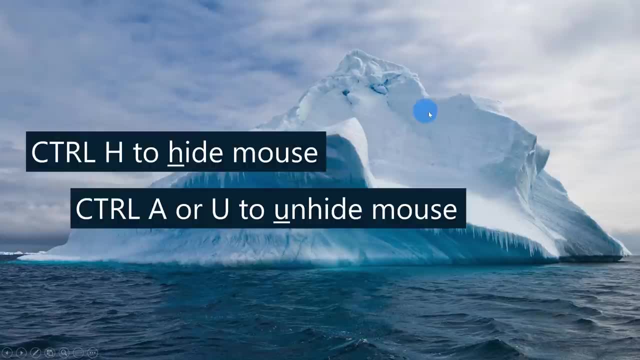 what language you want the subtitles to appear in. So there are some configuration settings that you have control over. Jumping into the next one, another nice one that you could use Right now. you see my mouse on the slide. Sometimes you don't want your mouse to appear, and so what you do is if you press control. 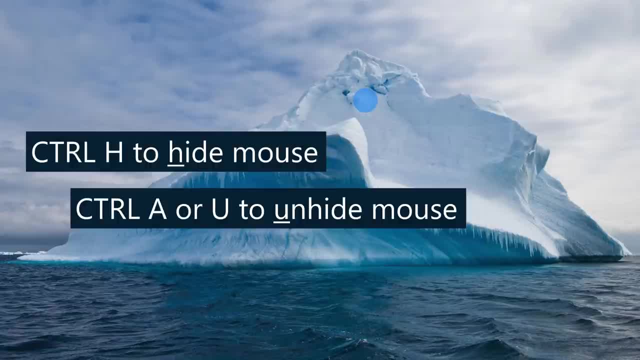 and H at the same time. So I'm going to press control and H. You'll see that my mouse disappeared. Now, once again, I'm using this cursor highlighter so you do still see the halo around where the mouse would be, And the H stands for hide. 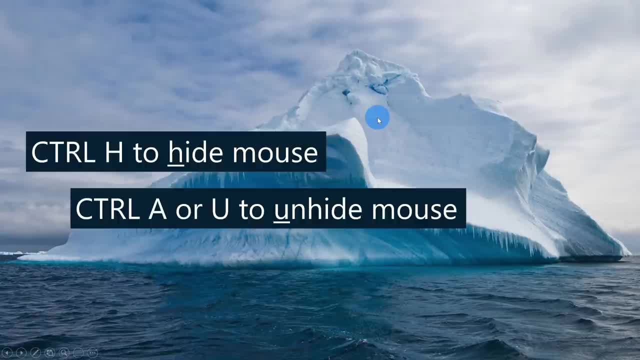 Now, if I press control A for arrow, that'll bring my cursor back, Or what I could do is I'm going to hide the cursor again. I could also press control U, and control U will also bring my cursor back. There it is. 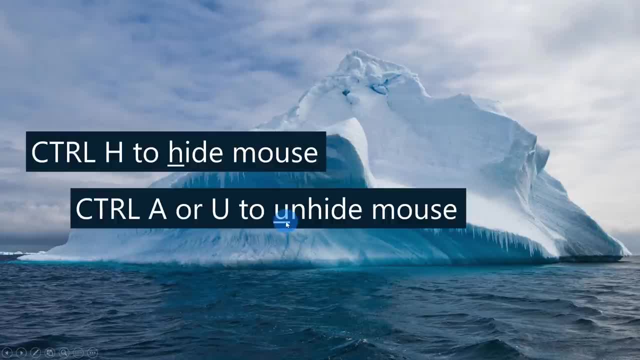 So both of those ways bring my cursor back And the? U goes along With unhide, so that's one way to remember it. Or control A. A is arrow. That's another way to remember to bring your cursor or your arrow back on the screen. 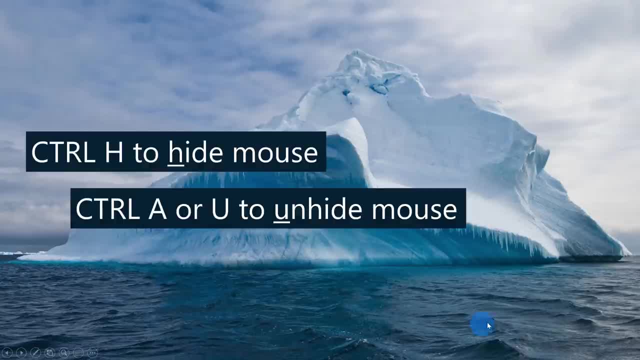 And I have a big iceberg in back because much of it is hidden under the water. You only see, I think it's something like a tenth of the iceberg is above and then nine tenths is below the water. So just went along with this hiding and showing. 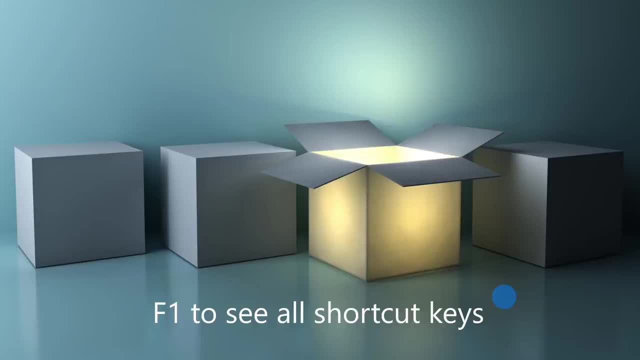 Okay, and then I went through all of these different shortcut keys. If you don't remember what they are, The one that you should remember- And the one that will unlock all the others- is pressing the F1 key. F stands for function. 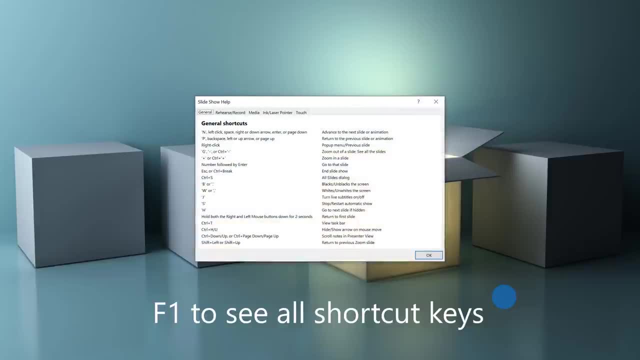 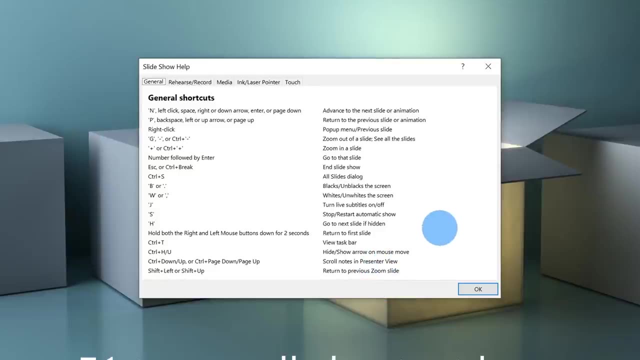 Those are the keys on the top of your keyboard, And if I press F1, what that'll do is it brings up slideshow help, And here I can see all of the different shortcut keys, All of the general shortcut keys. These are likely the ones you'll use most often or have to do with navigation of the. 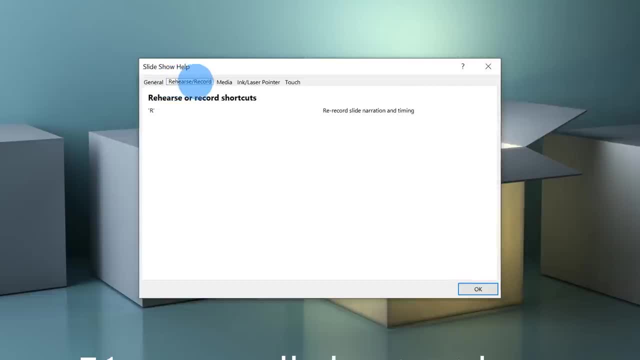 slides. You also have a set of rehearse and record shortcut keys that you could use. You have shortcut keys related to media. Let's say you have a video, You have a video embedded in your PowerPoint presentation or you have a song. You could use these shortcut keys to control that. 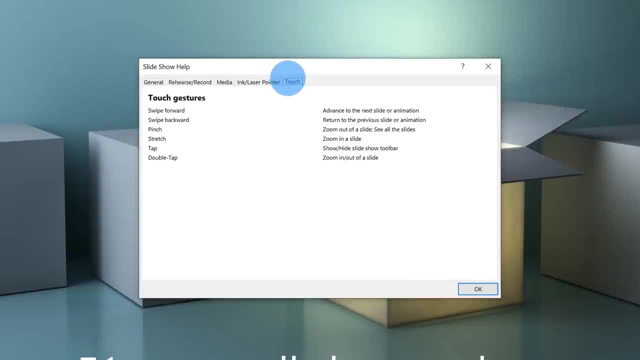 You also have all of the ink and laser pointer shortcut keys which we ran through. And then, lastly, if you have a touch display, you could also use gestures on your keyboard, or if you have your touchpad, you can use these different gestures to advance or zoom. 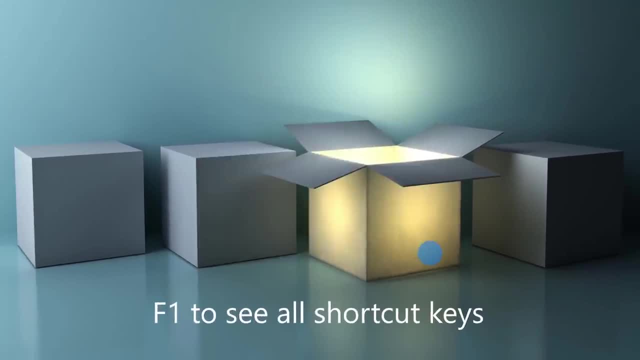 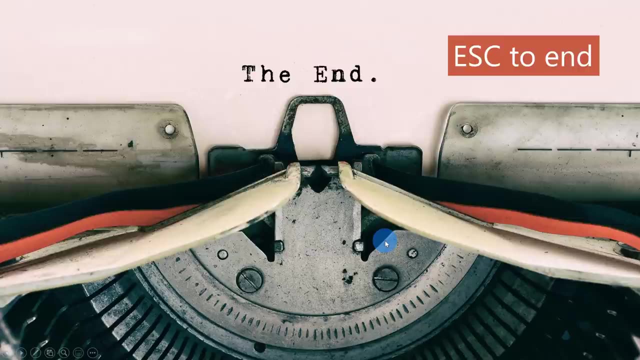 in or zoom out on your presentation. So I'm going to go ahead and let's click on, okay, And that brings us to the end of this presentation, And it all comes down to this. It also brings me to the last shortcut key that I want to share with all of you. 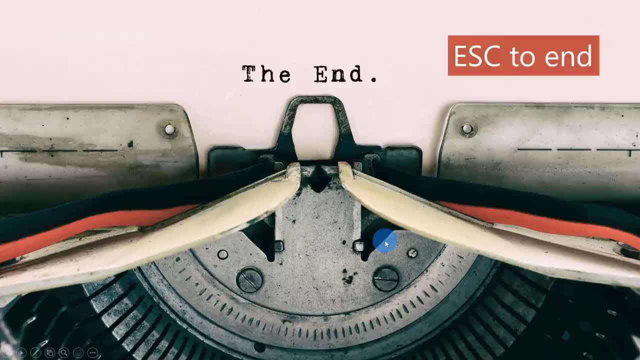 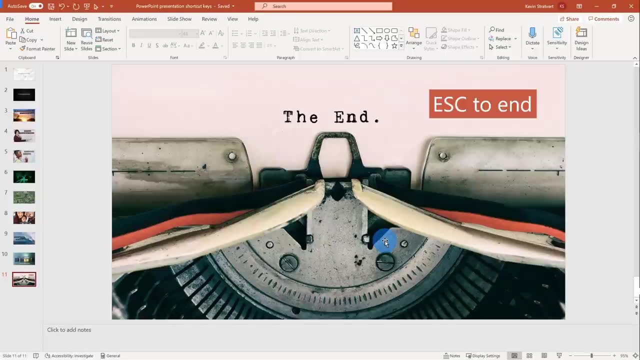 When you reach the end and you want to exit your presentation, simply press the escape key and that will bring you back into PowerPoint, And that is the last shortcut key that I wanted to show Now. we went through this presentation and I had lots of very beautiful imagery and it. 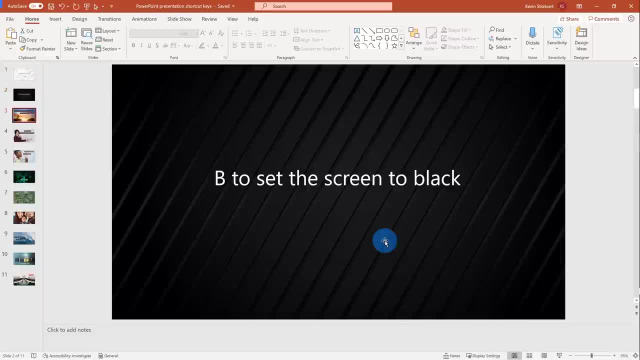 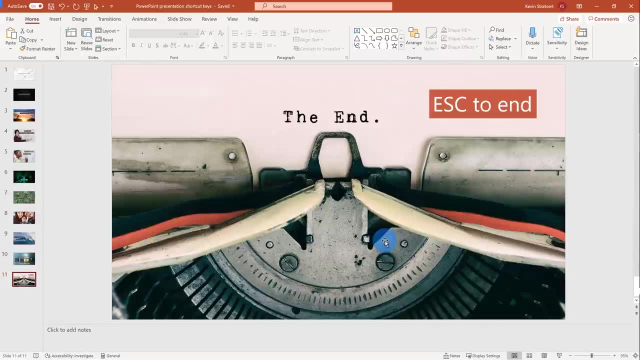 did not take me long to insert this And, best of all, all of these images that I used. these are royalty free. I could use them in my presentation without any problem, And I want to show where I got these from, So, within PowerPoint, this is something new that was added recently. 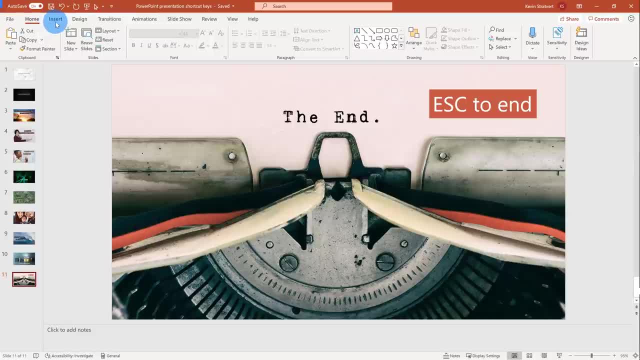 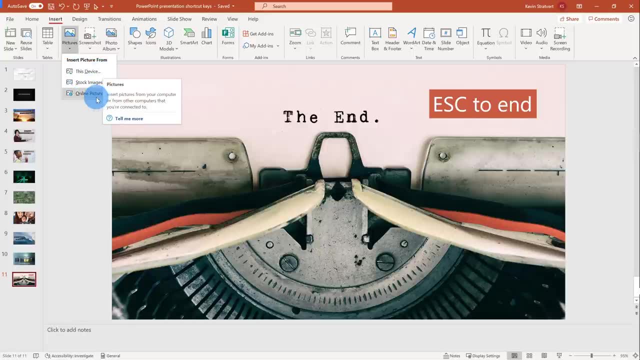 If I go up onto these tabs at the top or the pivots, I'm going to click on the one that says insert, And if I go to pictures, in the past I've been able to insert pictures from my device or online pictures. 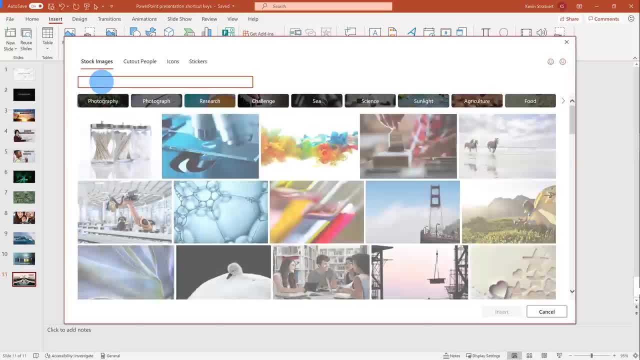 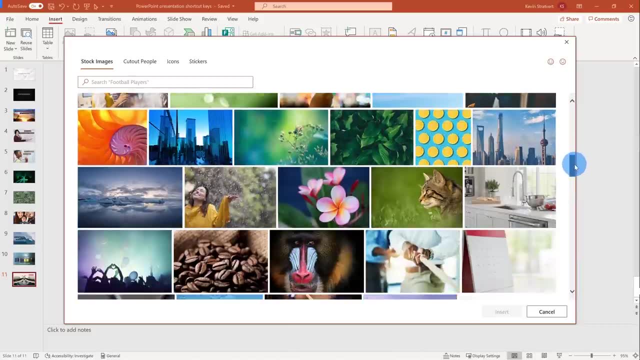 There's now a new option called stock images. If I click on stock images, this allows me to insert royalty free images into my PowerPoint presentation, And you might even notice These are the images that I used in my presentation. Now, the nice thing is, you could also search for different images. 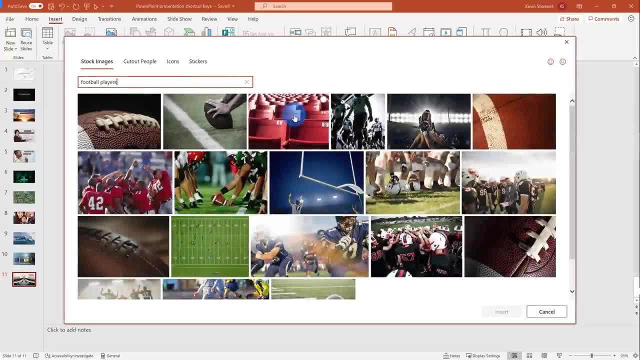 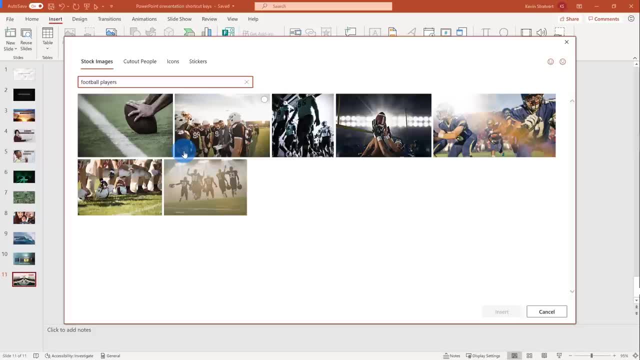 So I'll type in football players. That was one of the suggestions. If I type in football players here, I see all of the stock images related to football players, So search will help me find images that relate to whatever my slide content is on.